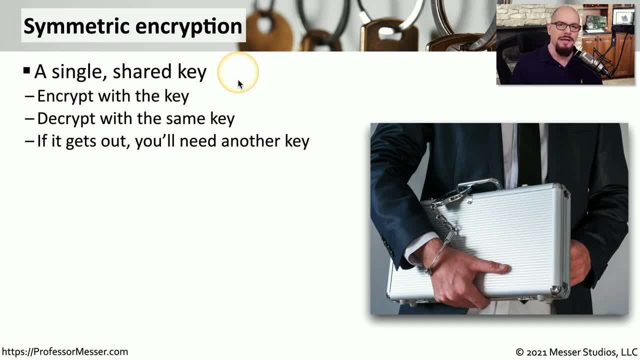 that you'll have to completely redo all of your encryption, because now everyone has a copy of the key that can be used to decrypt this data. You'll sometimes hear symmetric encryption referred to as a secret key algorithm or a shared secret. That's because that single key is the secret that 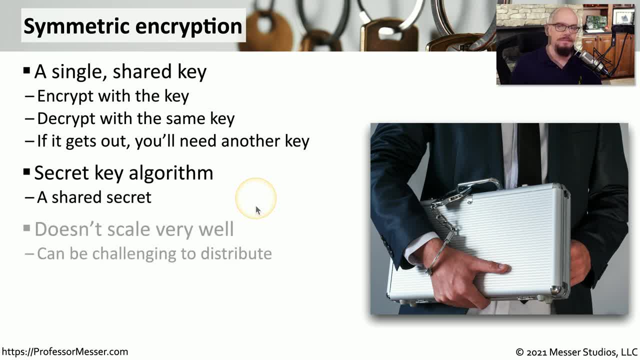 everyone needs to know to be able to decrypt the information. One of the challenges you have with symmetric encryption is it's difficult to scale. How do you share a key with others when you don't currently have a key? How do you share a key with others when you don't currently have a key? 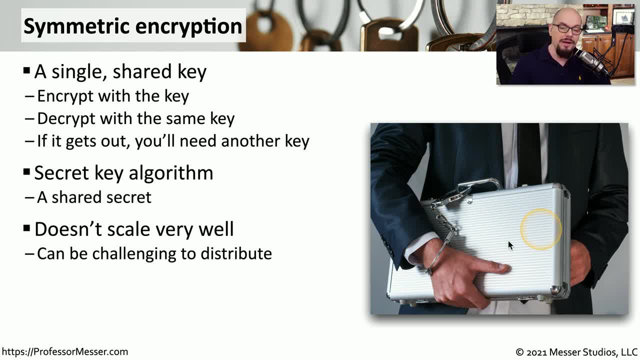 You can think of this as somebody carrying the key in a locked case. They're protecting the key until they get to their destination and only then can they share that key with another person. But across the network you don't have a locked case And since you don't have a key, that both 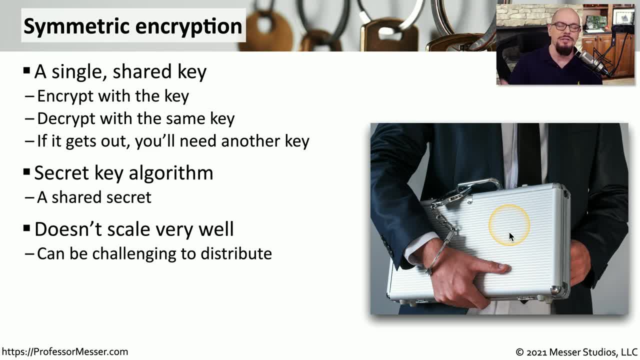 sides can share, you don't have a way to encrypt the key to be able to send it to the other side. This means we have to find other ways to be able to share this key so that we can use symmetric encryption. One way to get around this problem of scalability is to use asymmetric encryption. The problem 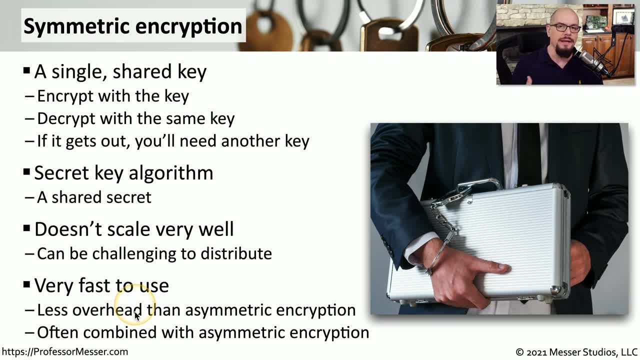 though, is that asymmetric encryption requires more overhead and more work by the CPU. Symmetric encryption requires relatively fewer resources than asymmetric encryption. Often you'll see the two combine, where you'll use asymmetric encryption in order to transfer asymmetric key to someone else. So very often those two algorithm types are used in conjunction. with each other, So that's a good way to get around this problem of scalability. One way to get around this problem of scalability is to use asymmetric encryption. The problem, though, is that asymmetric encryption requires relatively fewer resources than asymmetric encryption, So that's a good way to get around this problem of scalability. 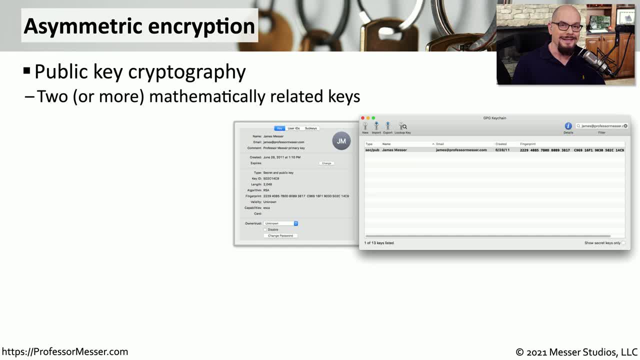 Unlike symmetric encryption, where there is a single key, with asymmetric encryption there are multiple keys. You'll sometimes hear this referred to as public key cryptography, because there is a public key and a private key. In some situations, there can even be more than. 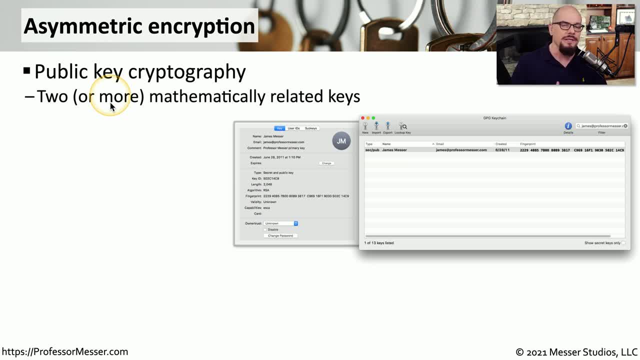 two keys, But for the examples that we'll give today, we'll deal with the two keys: a public key and the private key. The private key, as the name implies, is a key that only you have access to. So if you have a private key, you can use the private key as a public key. But if you 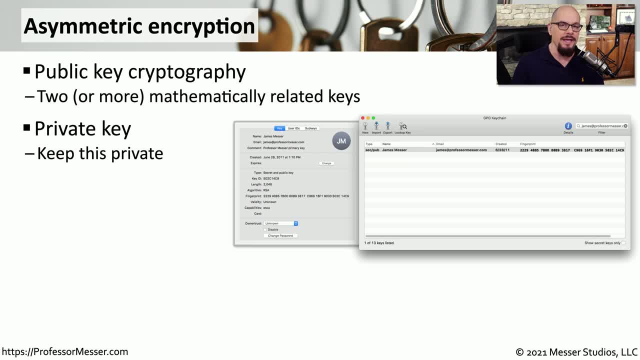 It is a private key because nobody else knows what that key is. There is another key that is mathematically related to the private key, called the public key. This is the key that you give to everybody. You can post the public key on a public key server. You can hand it out to people in email. 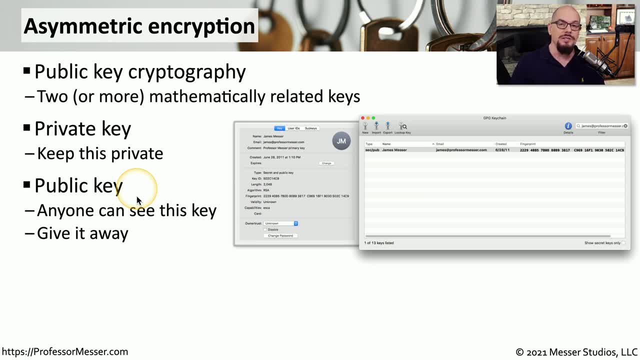 messages. You can put it on your website, And everyone who wants to be able to encrypt information and send it to you needs to have your public key. Once somebody encrypts data with that public key, the only way to do that is to use a public key. So if you have a public key, you can post it on. 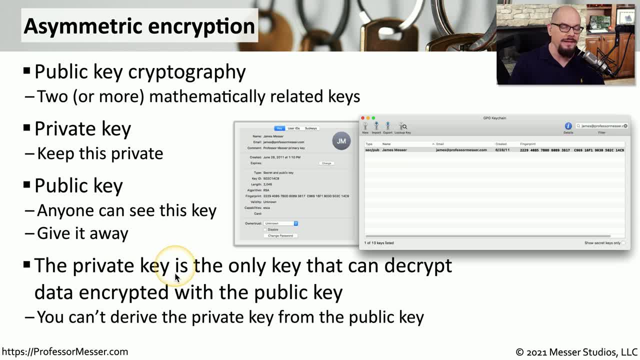 your website. You can decrypt that information is by using the corresponding private key, And, of course, that's a key that only you have access to. Interestingly enough, you can also do this the opposite way: You can encrypt information with your private key And the only people that would 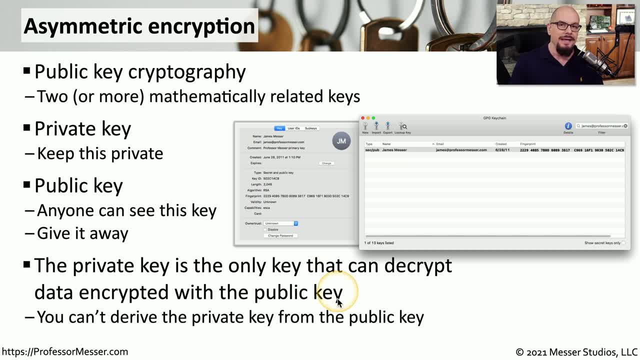 be able to decrypt it are the people that have the public key. This is the process that we would use for doing something like a digital signature, for example. So, although we've named these keys public and private, they're really only named that way because that's how we're going to decrypt it. 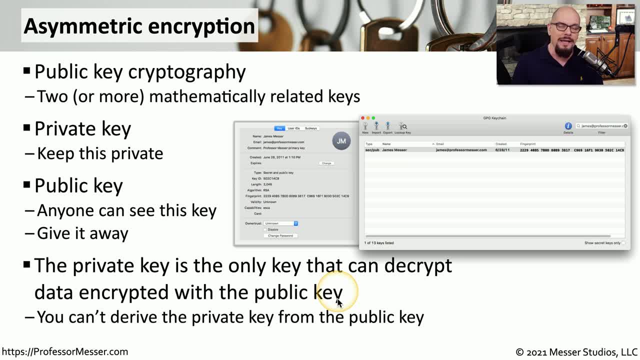 And that's how we're using them. The two keys are mathematically related And, depending on which one you choose when you create, the keys is the one that becomes the private key and the one that becomes the public key. Although these two keys are mathematically related, you still can't derive. 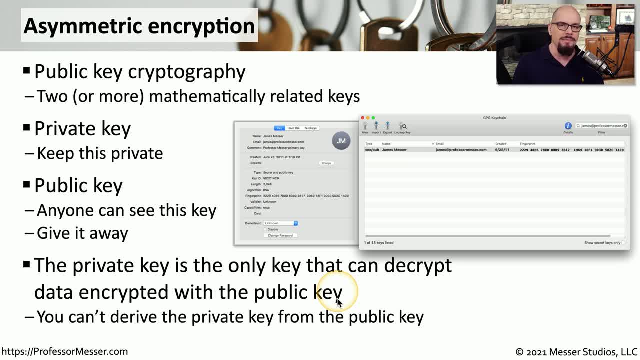 one key from the other. If everyone has access to the public key, they still would not be able to determine what the private key should be, even though they have full access to every part of the public key. It's this interesting relationship between the public key and the private key, And 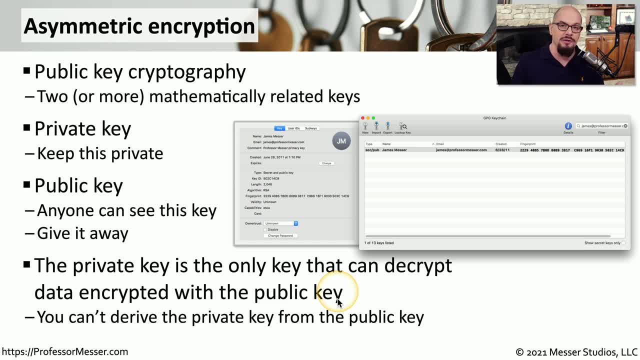 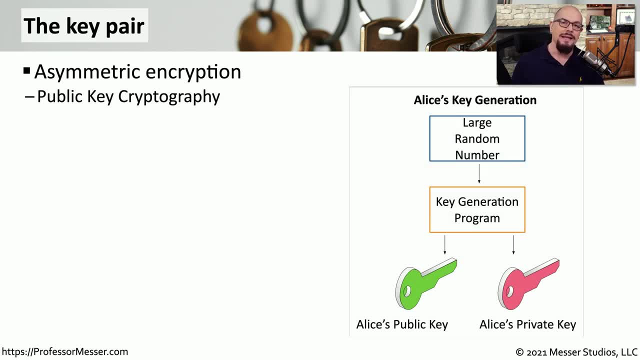 it's this interesting relationship between the public key and the private key that enables us to use the encryption that we have today on the internet. To better understand this relationship between the public key and the private key, let's go back to when we originally create this key pair. when using 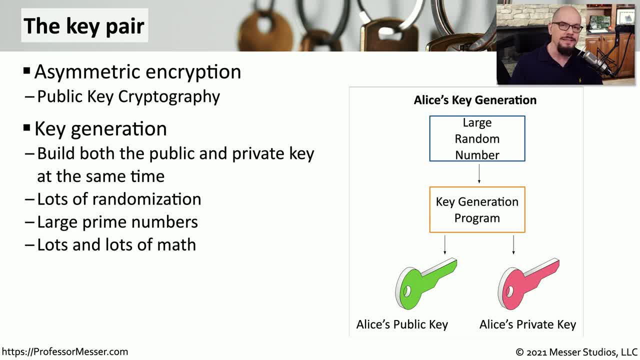 asymmetric cryptography, We would build both of these keys at the same time. We have a large random number. There's a key generation program that is input, And the output to that program creates the two keys- the public key and the private key, And we would build both of these keys. 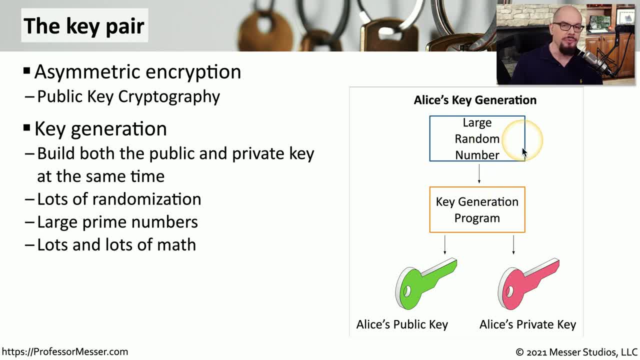 and the private key By running this key generation program, which uses large random numbers and prime numbers as input, it runs it through a generation program and it outputs two separate keys. Of those two keys, we choose one of them to be the public key and one of them to be the private key. And 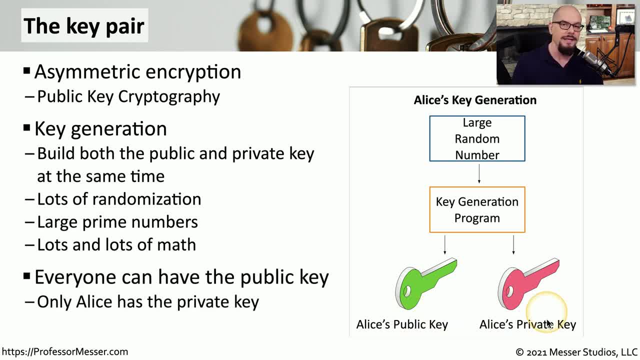 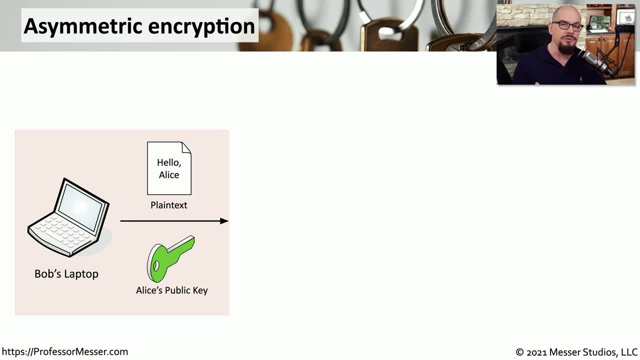 then we share the public key with everybody and we keep the private key private to us. Let's look at the process that's involved in encrypting and decrypting information using asymmetric cryptography. Let's look at the process that's involved in encrypting and decrypting information using 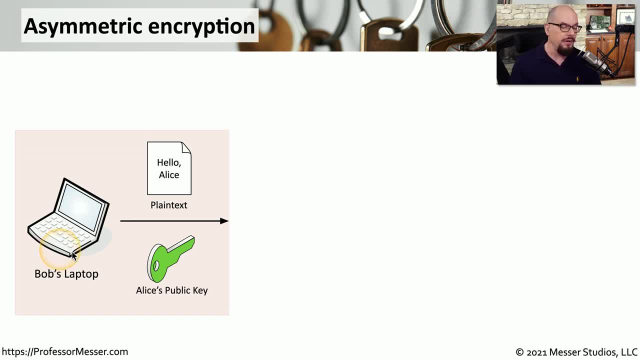 asymmetric cryptography. Let's take a scenario where Bob and Alice are communicating to each other and Bob would like to send some information to Alice that is encrypted. Bob will need a way to create this encrypted message like a laptop. He'll need the original plain text. This plain text says: 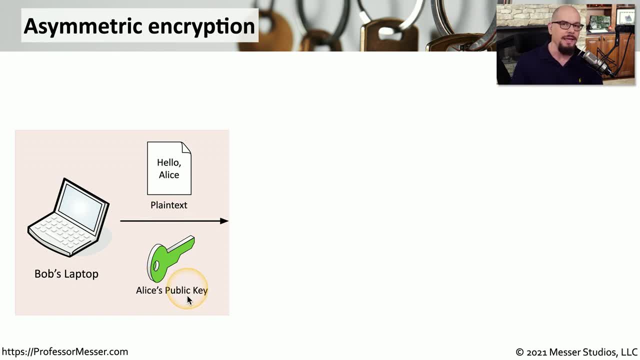 hello Alice. And then he'll need Alice's public key To obtain this key. Bob can ask Alice for her public key. He can retrieve her public key from a public key server, or he can visit Alice's homepage or anywhere else. Alice may have posted the key. Alice may have posted the key to Alice's. 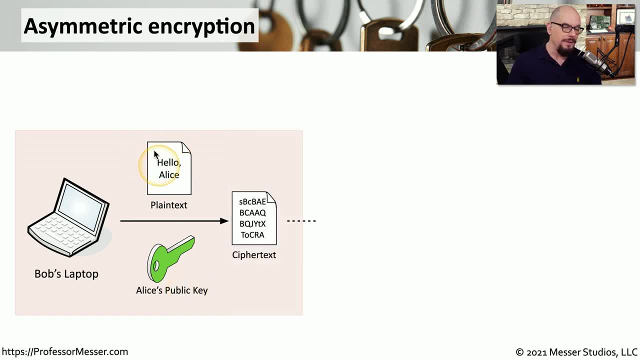 and download the key from there. Bob then combines the plaintext with Alice's public key to create the ciphertext. Once the ciphertext has been created, the only way to obtain the original plaintext is to decrypt it with the private key. You cannot use the public key to somehow undo the encryption. 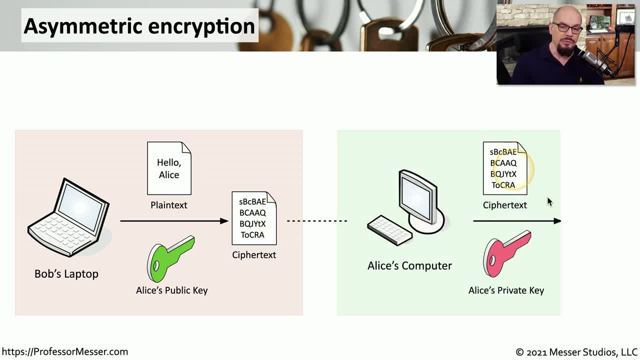 process that you've already done. This means that Alice will receive the ciphertext message and will apply her private key to be able to decrypt that ciphertext And once that's decrypted she'll be able to see the plaintext that says: hello Alice. 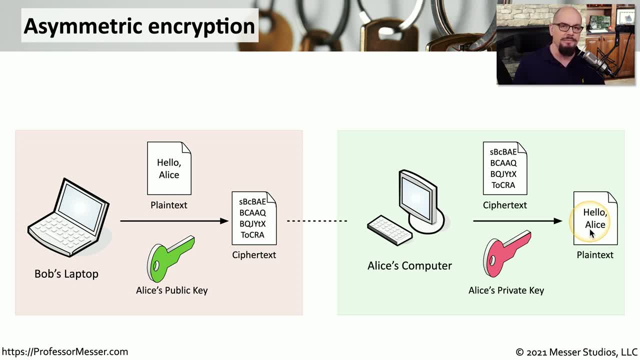 This is the process that occurs every time someone wants to send information using asymmetric encryption. If we wanted to reverse this process and have Alice send encrypted information to Bob, she would need Bob's public key, she would encrypt the data, send that ciphertext to Bob and Bob. 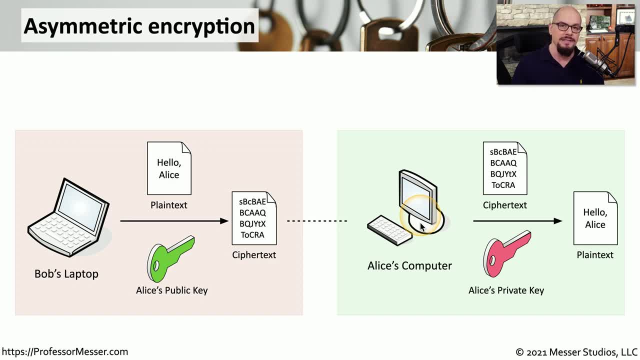 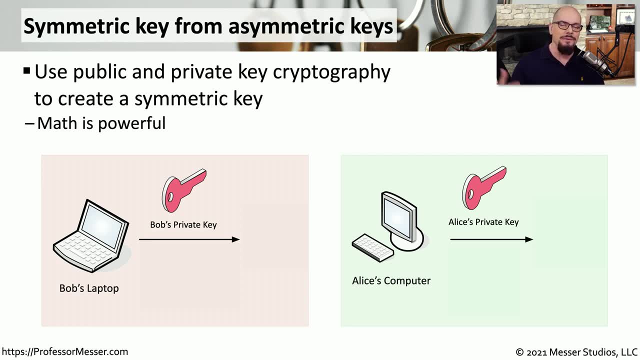 would use his private key to decrypt that ciphertext. We spoke earlier of the difficulties in being able to scale a symmetric key, because there's no easy way to transmit that symmetric key across the network without first encrypting it. And since you haven't sent the key across the network, 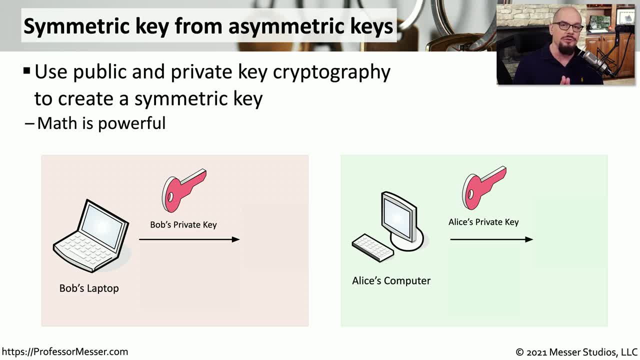 there's no way to have a known key on both sides that you can use for the encryption process. One way to get around this problem is to use asymmetric encryption in order to create a symmetric key on both sides without having to send that symmetric key. 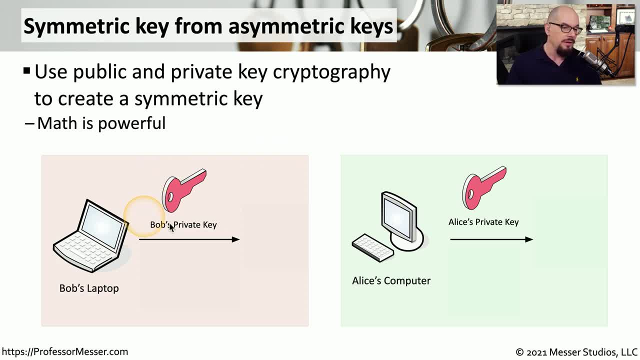 If you want to do that, you can use the public and private keys on both sides. Let's take the example again of Bob and Alice. We know that Bob and Alice use asymmetric encryption, which means that Bob has a private key and Alice has a private key. 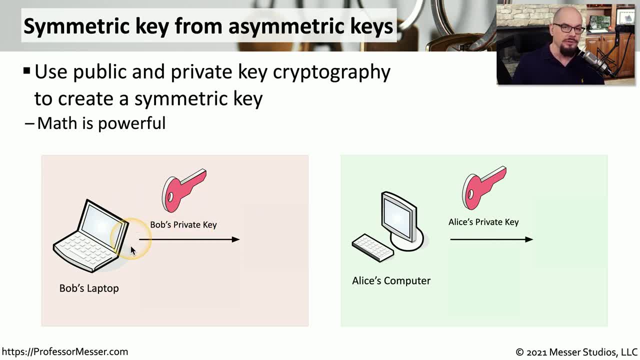 And, of course, those private keys are only known to their owners. You can combine your private key with someone else's public key to create a symmetric key, And if you use the related public and private keys on both sides, you end up with a symmetric key, that's. 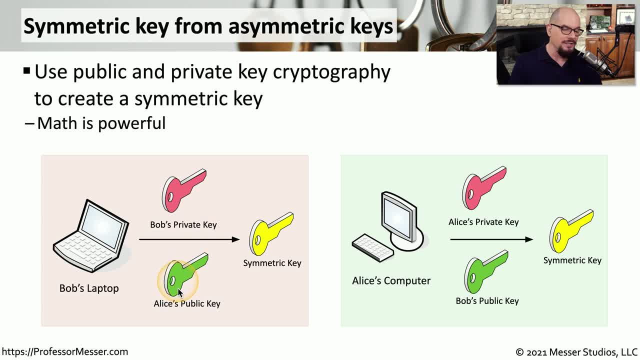 identical to each other. So, even though Bob's private key and Alice's public key created a symmetric key, it's exactly the same symmetric key if you combine Alice's private key and Bob's public key. By doing this, the same symmetric key can be created on both sides of the conversation. 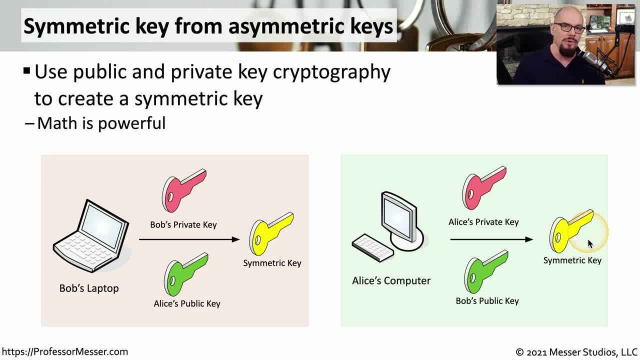 without ever having to send the symmetric key across the network. In fact, this is the process used for Diffie-Hellman key exchange And it's a key exchange. It's a key exchange process that's used extensively every day. Hopefully you're starting to see. 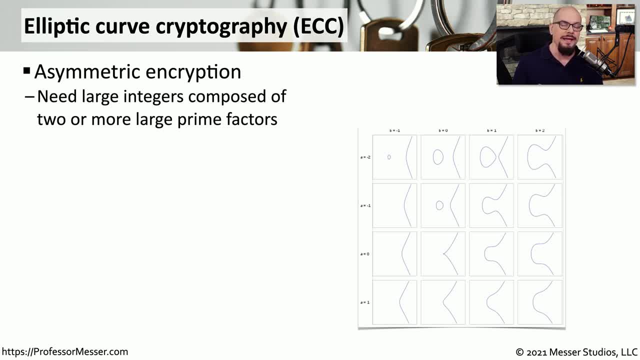 that asymmetric encryption can provide us with functionality that symmetric encryption simply can't do. But there are some drawbacks to using asymmetric encryption. We're using very large integers of very large prime factor numbers And that calculation requires CPU overhead and resources on a machine to be able to encrypt and decrypt. 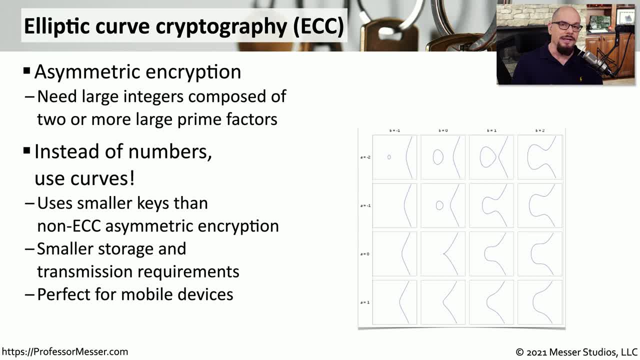 that information. Of course, we have mobile devices and Internet of Things, devices that may not have the computing power that our local workstations have, but they still need to be able to encrypt and decrypt information. For those, we would use elliptic curve cryptography or ECC.